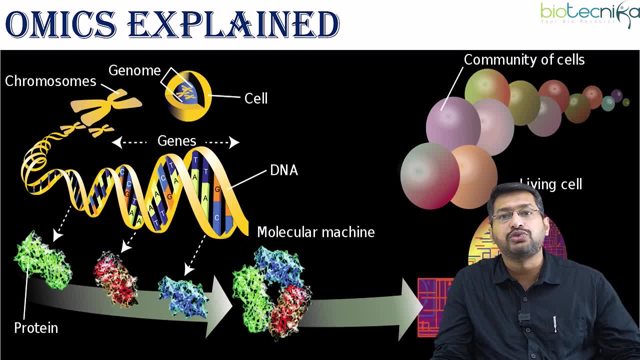 arranged and hence a new terminology called omics was being, you know, generated, or it was being coined. So let us try to see what are the various kinds of omics which are normally used in terms of bioinformatics and other data sets at large. Now, before I go into omics, let us try to also understand the basics of molecular biology or cell biology. Now, if I take up a cell, give me a minute. So, if I take up a cell, give me a minute. 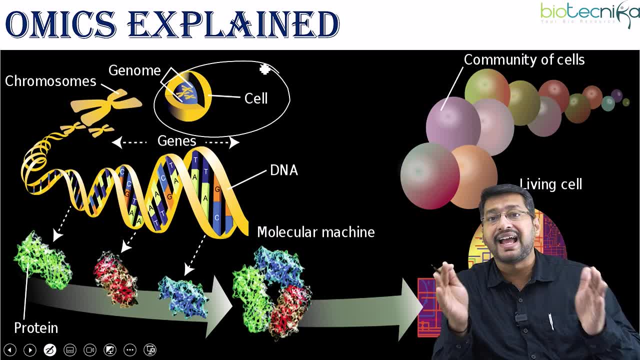 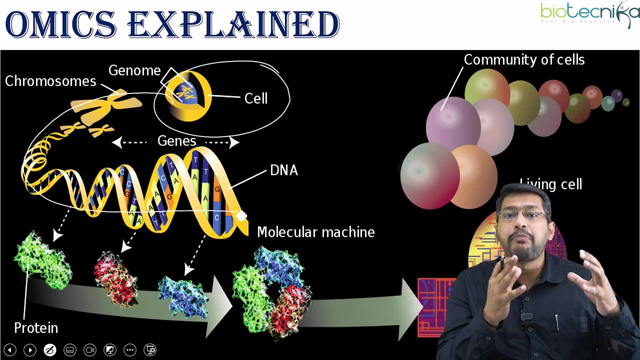 up a cell. so this is a cell, and from a cell I have a nucleus and inside the nucleus I have chromosomes. Now if I open up this chromosome in a nucleosomal model, I get the proteins and the nucleic acids. So the nucleic acid has been bound with a set of proteins which are normally called. 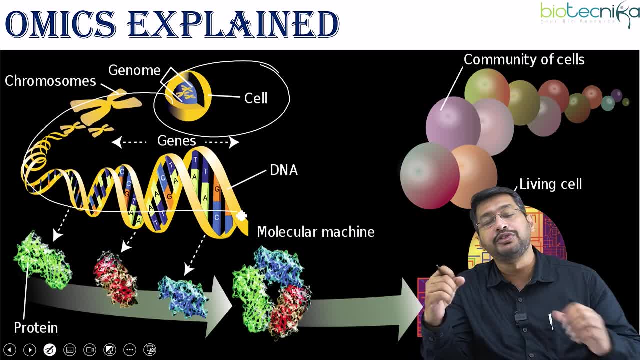 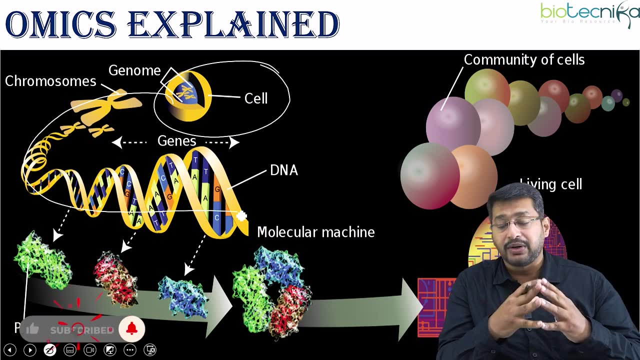 as histones. and then you have the other set of nucleic acid, which is the DNA. Now, this is a combination of protein, and nucleic acid makes a complex structure to actually store a huge number of data, what we call in terms of nucleotides and nucleosides. Now, using all these molecular 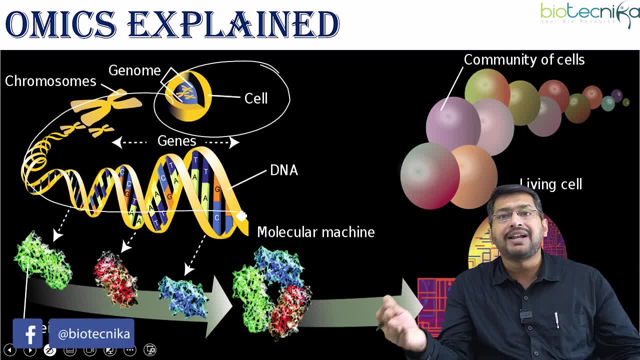 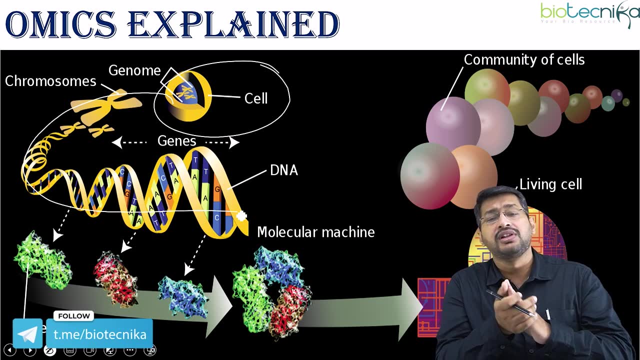 machinery. what people thought is: why don't I apply technology onto it, okay, and then try to see what advances can I still make in terms of this omic approaches. So people thought of integrating electronics with- especially in electronics, that is, microelectronics- Microfluidics with that of molecular biology, and now they have created a beautiful system. 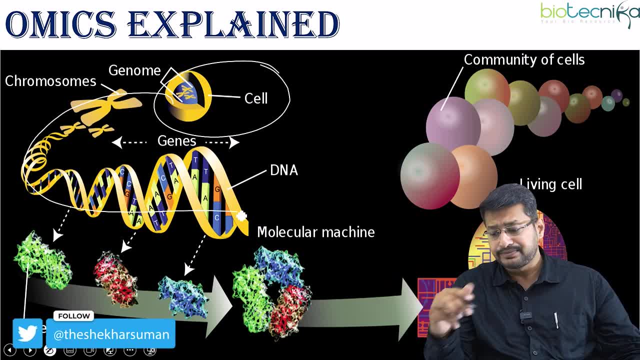 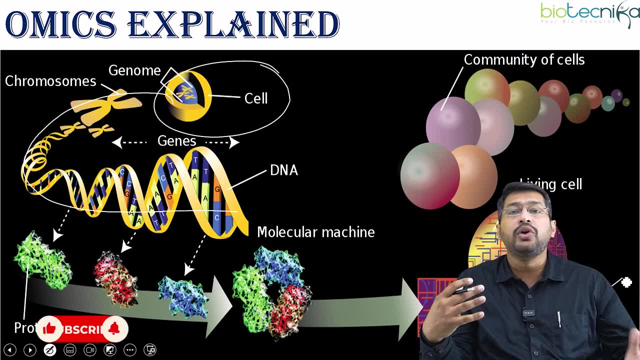 which is called as organ on a chip or human on a chip. So if you look into this slide or the circuitry, so this circuitry talks about the entire metabolism which is going upon in a cell, and then I can still looking into the circuitry and the various impulses which have been generated. I can 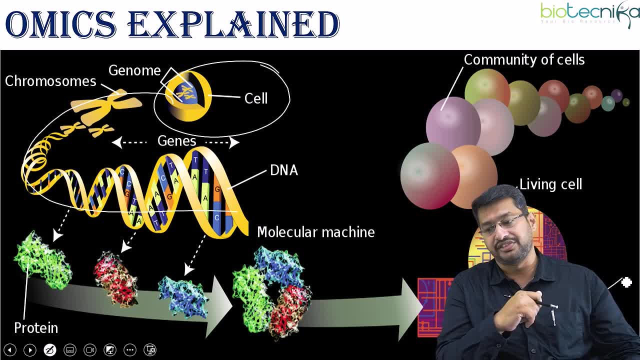 tell a given patient is suffering with what kind of diseases or disorders. and that's again in terms of regenerative medicine. people are also talking on the communities of cells, wherein how do I create totipotentic cells, how do I create pluripotentic cells and how do I create, you know? 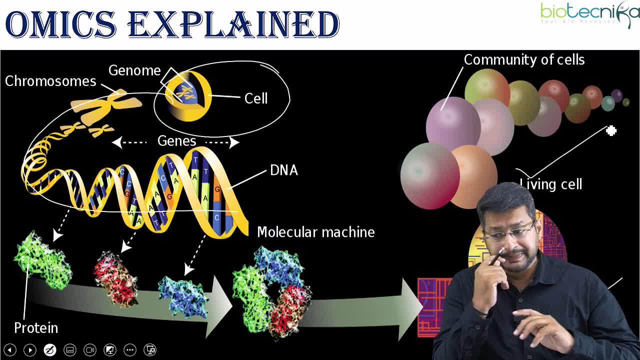 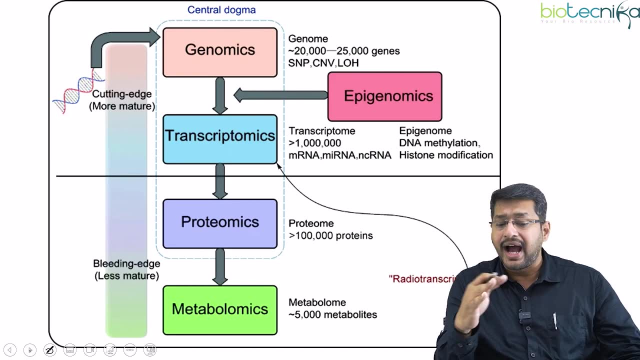 you know lymphoidal cells. So in all these conditions, you know new, new terminology. every day new, new terminology is getting you know, eluded, and let us try to see what exactly are these new terminology. I'm sure that you know, you, everybody in molecular biology knows the central dog of molecular biology. 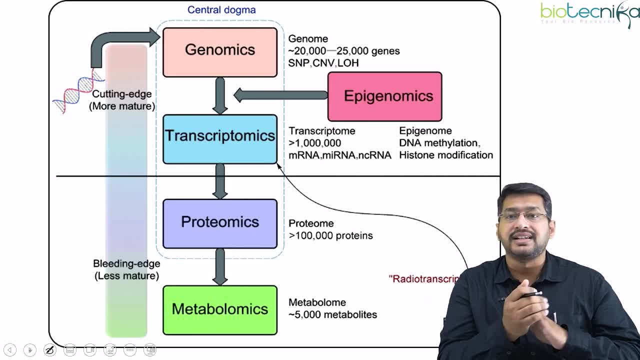 which starts with the two different components. one is called as the classical central dogma, cosa planetary, and the second one is called as the modern centered dogma of molecular biology. so if you look into this particular pathway here, if I look into this particular pathway, so this particular 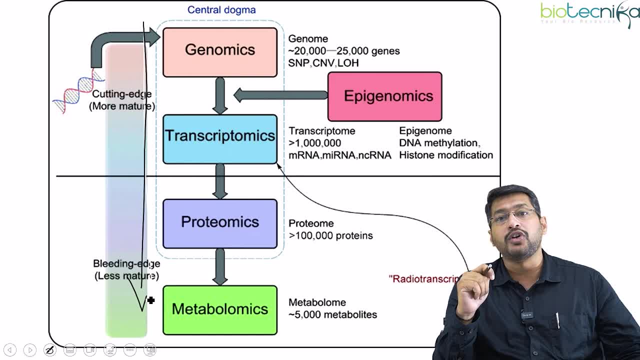 pathway refers to the classical central dogma of molecular biology. biology started with the DNA, DNA getting transcripted into RNA and RNA getting translated into proteins. So the study of the DNA was coined as genomics, The study of RNA and its regulation was termed as transcriptomics, and the study of 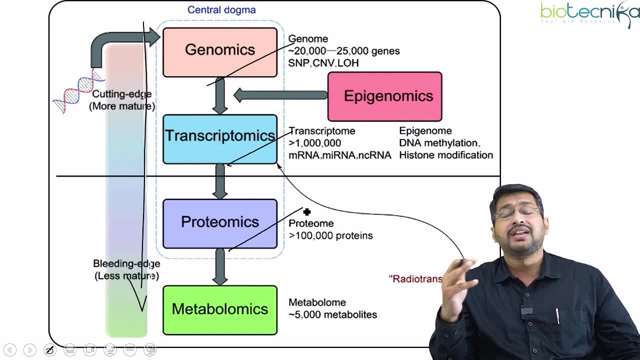 proteins was called as proteomics. Now, for the last 10 years, you know this- genomics, transcriptomics and proteomics was the only three terminologies which was used in the central dogma. But, however, because of more amount of science and more amount of data, people thought we cannot just 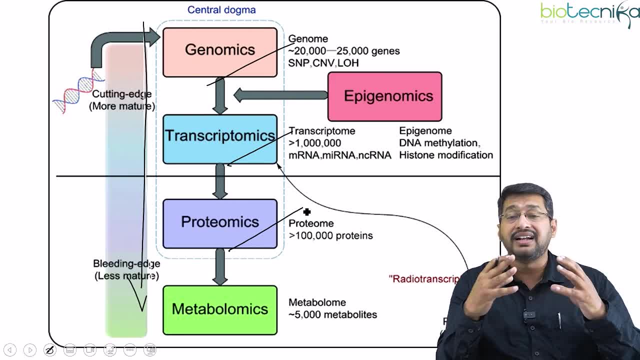 restrict the central dogma only for these three components and hence a two more new components were added, And these two more components were labelled as epigenetics and then metabolomics. Now, what are epigenetics? So epigenetics or epigenomics? 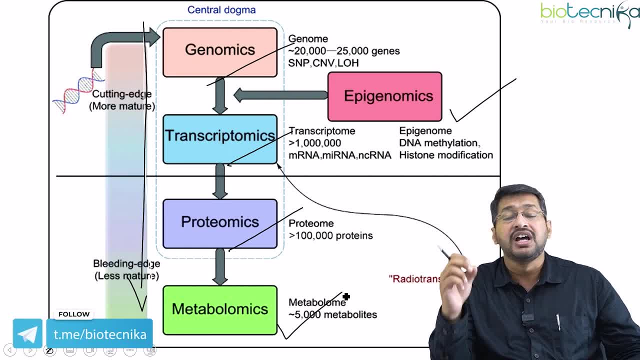 bee Nazi monster is a branch which talks about certain factors which actually control the DNA. so factors such as miRNA, factors such as HDACs, all these are factors which are in turn controlling the DNA replication. so hence, you know, the generational characters, or the hereditary characters, has to 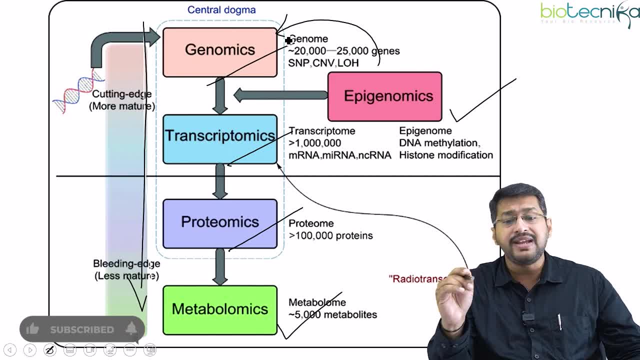 be studied at an epigenetic level and hence it has been very important in studying the various hereditary disorders and especially even in terms of autoimmune disorders. now people are trying to connect epigenetics and genomics and then trying to elude the association or the interaction between. 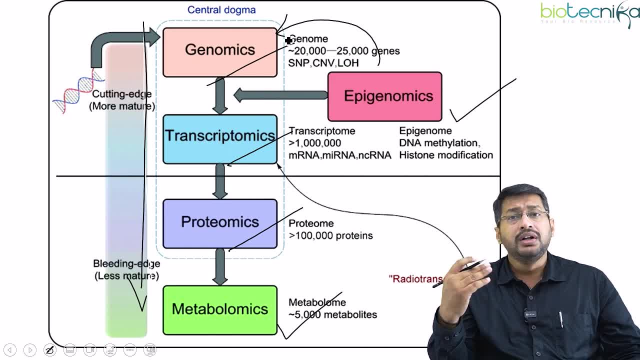 epigenetics and genomics. Now, what we have learned is epigenetic. there are certain factors, which we call it as epigenetic factors, which will control the DNA, and DNA will, in turn, gets transcripted into RNA and RNA gets translated into proteins. 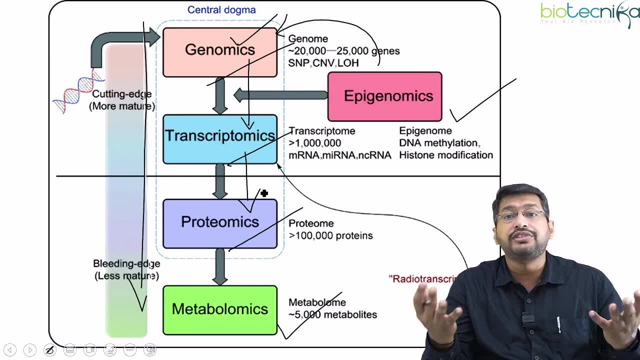 However, these proteins again, they undergo a process which is called as metabolism. there are various pathways. we have actually discussed this in our previous video. that is, we we spoke about metabolism, we spoke about anabolism and catabolism. Now, as a product of metabolism, anabolism or 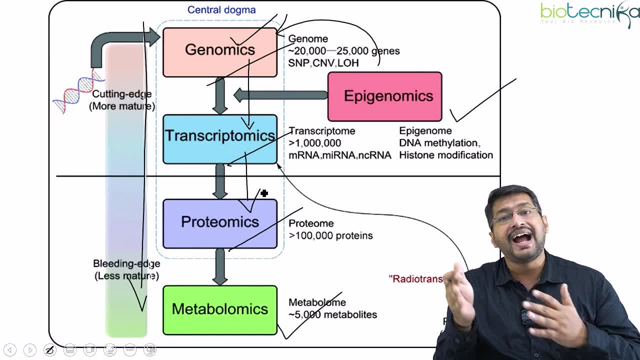 catabolism. we have metabolites, anabolites and catabolites. so in turn, I have a series of metabolites which could be either undergoing up regulation or down regulation, creating or actually limiting or determining the rate limiting step in a given reaction. and all these 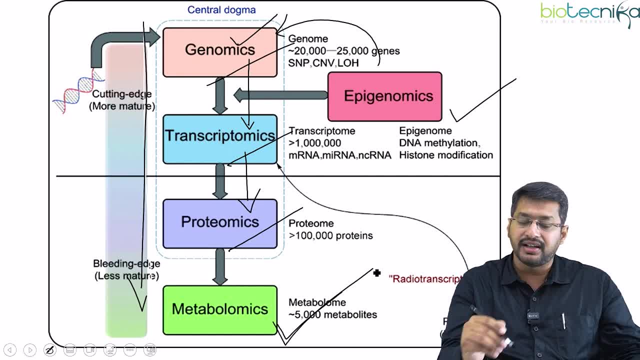 things are put into a special domain, and this domain is called as metabolomics. So what is the, the new central dogma, or the modern center dogma? it starts with epigenetics, from epigenetics it goes into genomics, from genomics it is transcriptomics, and from transcriptomics it goes. 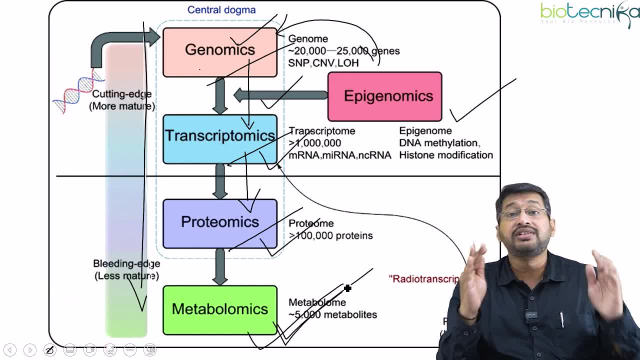 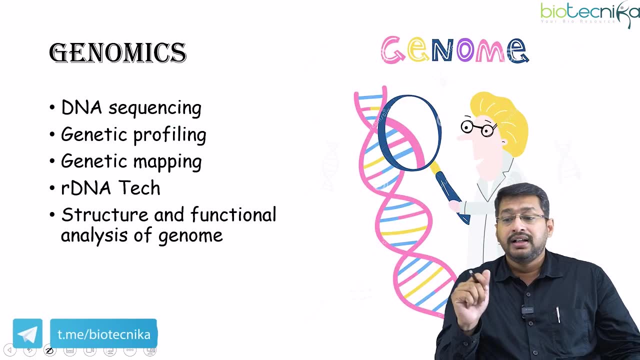 to proteomics and then goes on to metabolomics. So this is the major difference between the dogma of central- you know, central- dogma of molecular biology and the modern center dogma of molecular biology. Let's try to see the next slide Now. what do I study in genomics? So, as we have, 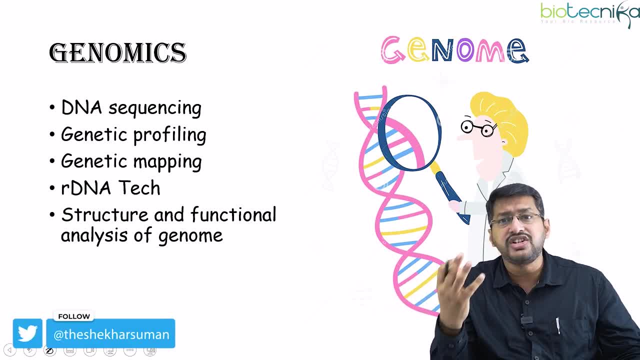 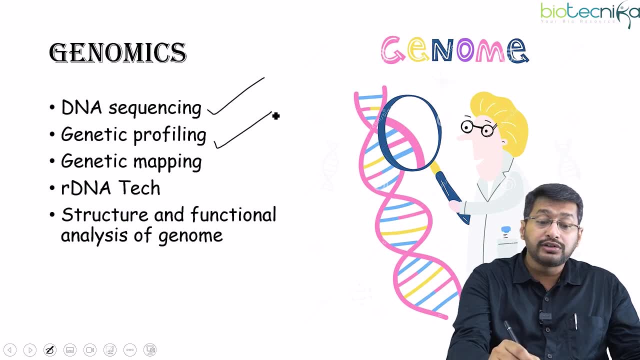 already seen that genomics is the the major concrete of studying DNA by doing DNA sequencing, by genetic profiling and also by mapping the genetic components and then our DNA technology and understanding the structure and functional analysis of the genome. Now genome is the entire complete set of genes are called a genome, and understanding the structure and functional. 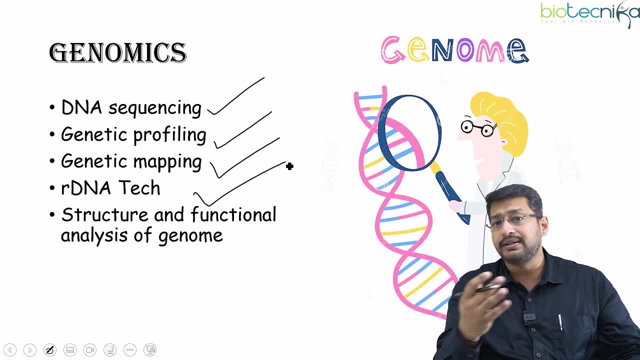 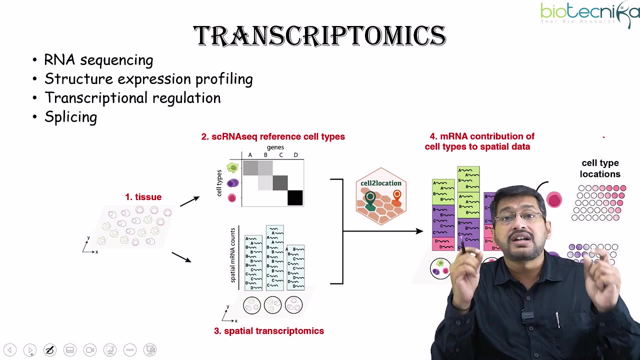 analysis of a genome might be from bacteria, might be from plant or from humans. so, depending on that, I have human genomics, plant genomics or bacterial genomics. so this is in terms of genomics. Now the next part is the transcriptomics. please remember the regulatory component I cannot study until 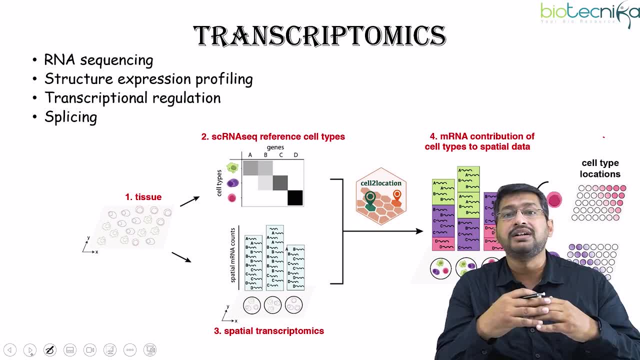 the end of this lecture. So what we do is for the regulatory component. we always rely on the RNA, and when we talk about RNA, it is the mRNA which is of a major use. So here, using transcriptomic analysis, it helps me to understand the gene expression profiling and also it helps me in 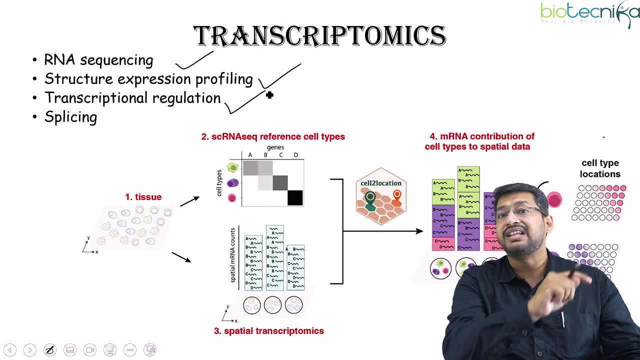 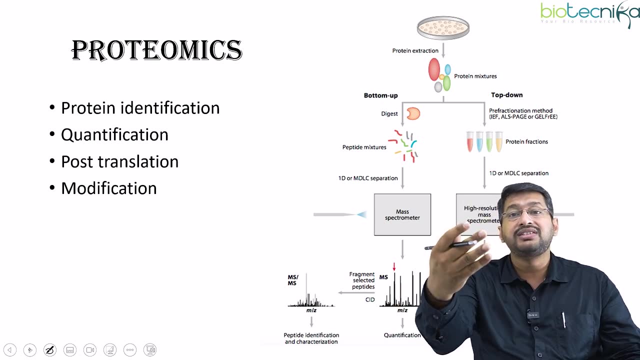 understanding the transcriptional regulators and master transcriptional regulators and, very importantly, the splicing mechanism which takes place between the introns and exons could be using transcriptomics. Now, what do I study in proteomics? Now, as we know, the data which gets a transcripted from transcription to translation, I have an end product and this end product is my. 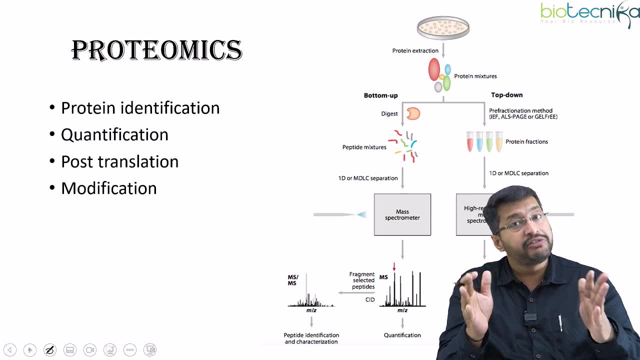 protein A very, very fickle molecule- okay, and very, very intelligent molecule. so this can actually create, can be a boon or also could be a bane. So here understanding this protein becomes very, very crucial for understanding and identifying the gene expression of the genome. So this is a very, very 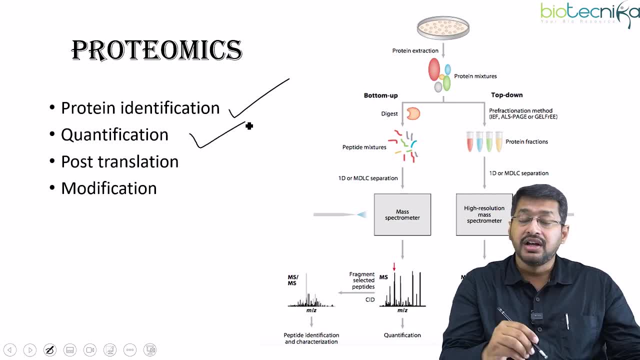 crucial for understanding and identifying the gene expression of the genome. So here, understanding this, this identification of proteins, quantification of proteins, very importantly, modification of proteins in terms of post-translational systems, becomes very, very crucial and hence, putting everything into this one umbrella is called as proteomics. 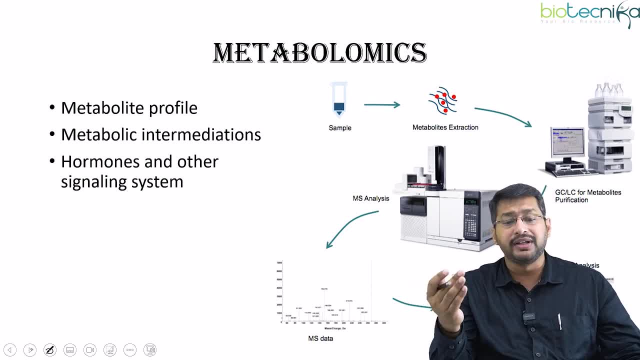 Then, as I you know, briefly described what exactly is metabolomics. In metabolomics, we are actually trying to profile the individual metabolite which could be either an handling or a catabolite, and we what are the various intermediates of metabolism which are being produced? 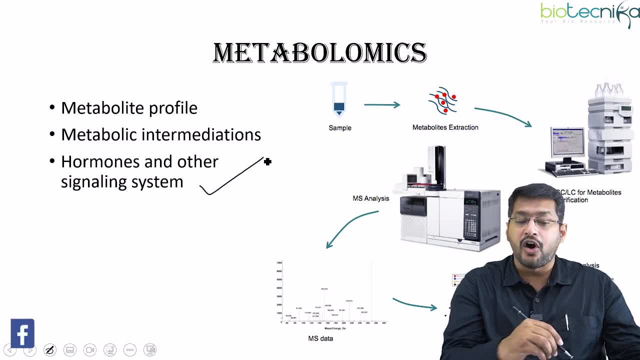 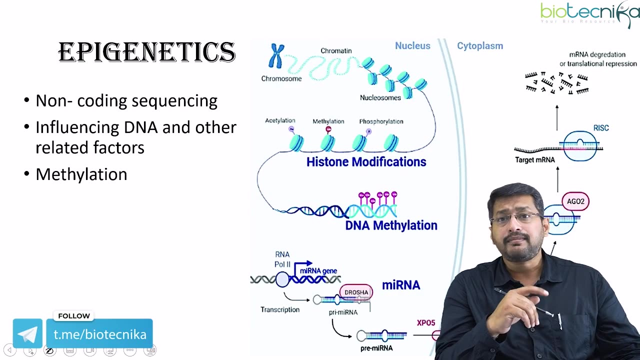 Now, when I talk about metabolism, we cannot exclude hormones and their signaling systems. So all the signal transduction systems comes under this particular metabolome, and the study of all this into one consortium is called as metabolomics. Now we also said that in central dogma of molecular biology 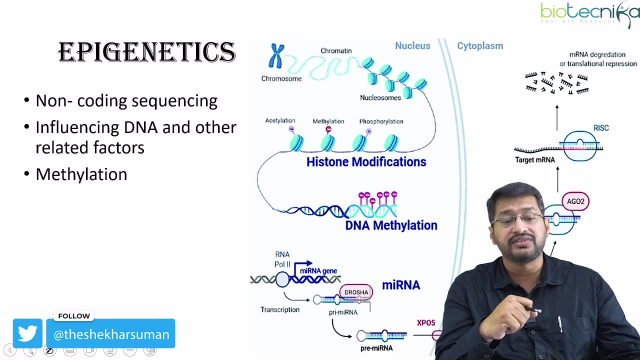 there is a new domain which is called as epigenetics or epigenomics, which mainly refers on to the non-coding sequences which are actually influencing the coding part, that is, the DNA. Then the influence and the related factors could be also studied. 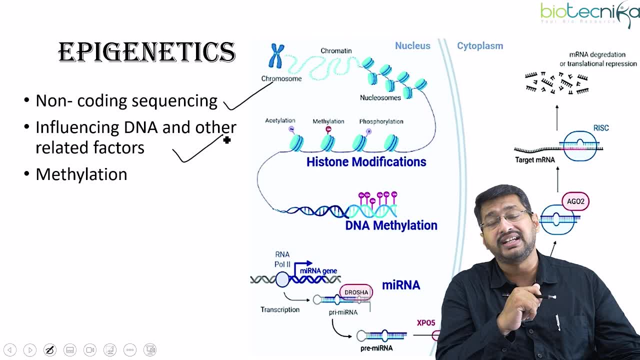 and very, very important modification which takes place on DNA. that is called as methylation. Now this methylation could be again predetermined by certain other factors, such as microRNAs- we also call it as miRNAs and HDACs. So all these play a very important role. 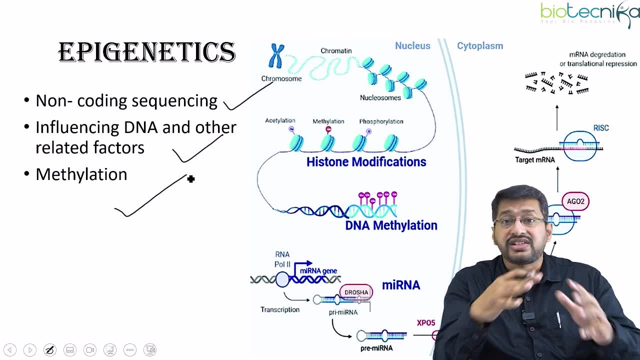 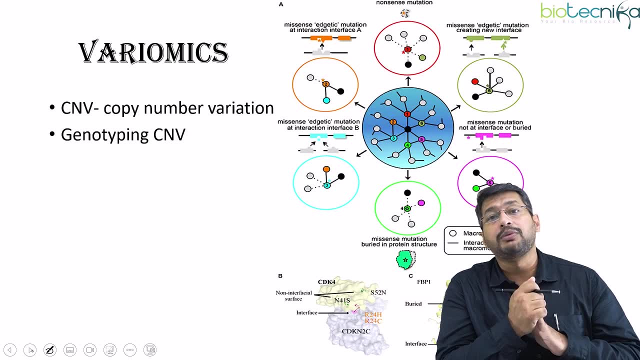 In the DNA methylation processes and studying this into one umbrella is called as epigenetics or epigenomics. Now, this was until, the central dogma of molecular biology. Now, as the data sets got increased. so for creating a perfect data set and to keep on adding much more data, 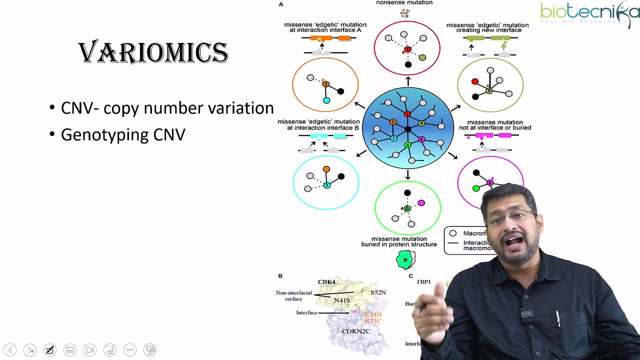 so what people thought was: let us try to create compartments, and these compartments have led into a new kinds of omics terminology. And let us try to see what are these new terminologies? So the first terminology is called as variomics. 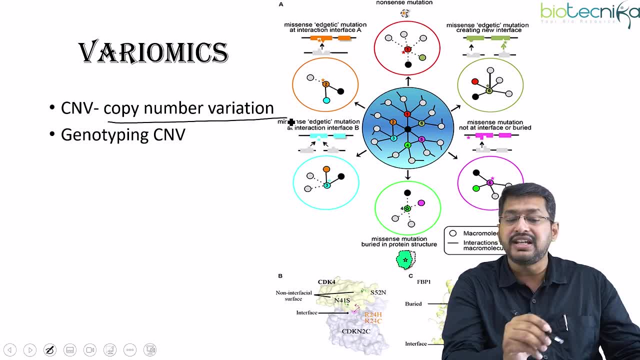 So in variomics we talk about the copy number variation, which is called as CNVs. So we talk about the copy number variation. and also in genotyping or ribotyping or in serotyping, we look into what are the variations at a molecular and submolecular or sub-submolecular levels. 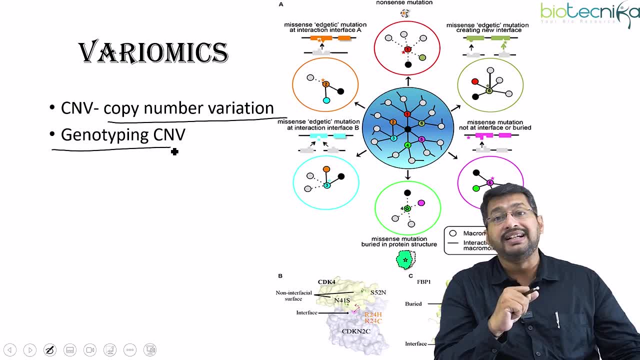 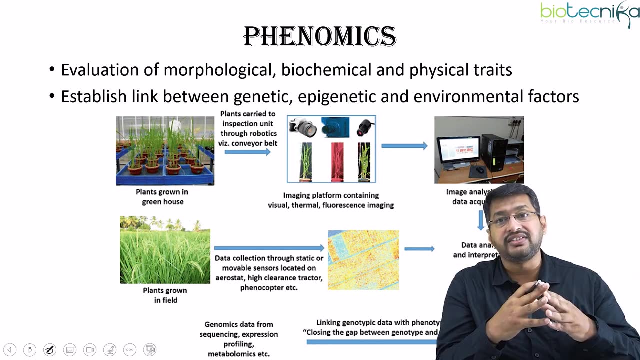 and these variations could be studied, becomes very, very important in disease diagnosis And treatment, and hence this comes into a newer umbrella, and this umbrella is called as variomics. The next terminology is called as phenomics. Now, since everything in genetics has been always dependent on the genomic component and the phenotypic characters, 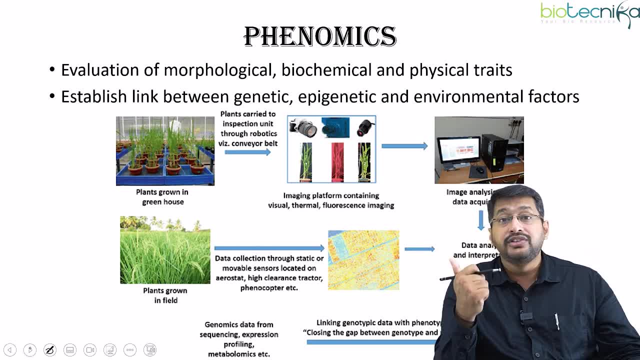 so studying the phenotypic characters, which includes the morphological characters, biochemical characters and physical trait of a given organism, and its evaluation is called as phenomics. So it creates a very important establishing link between genetics, epigenetics and, very importantly, environmental factors. 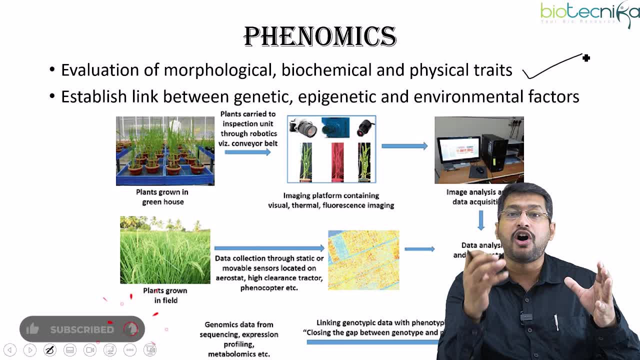 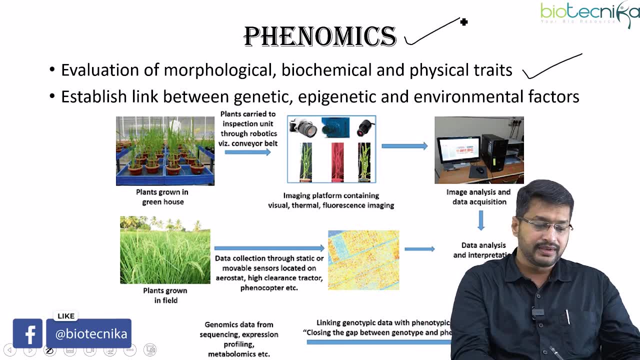 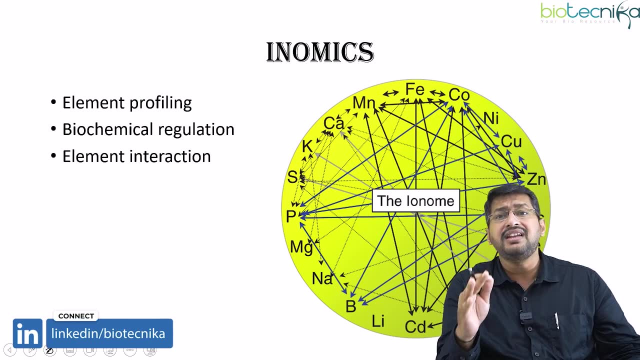 So here in phenomics we study a close association of an organism with its habit and its habitat, and this comes into a newer domain which is called as phenomics. Now the next one, and very interesting, is the ionomics. Now, in ionomics, as we all know that there are various kinds of metals and minerals which 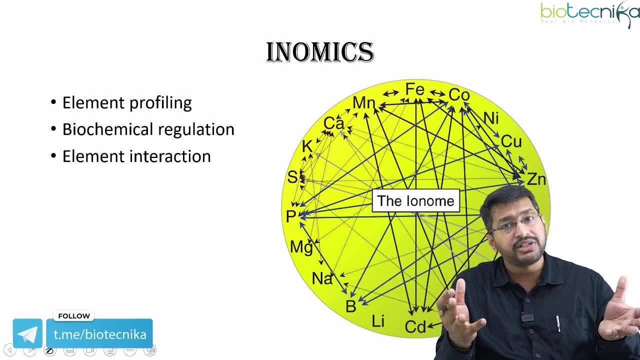 play a very, very crucial role, either in terms of enzyme activity or in terms of protein activity. Here we speak about the element profiling. the biochemical regulations on the involvement of these ions say, for example: you know, the presence of iron and its regulation in. 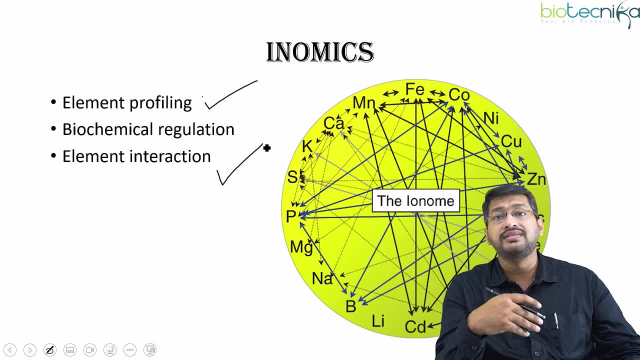 hemoglobin synthesis, or I can also talk about the zinc fingers, I can talk about the various elements which are actually interacting with a larger macromolecule or a larger biomacromolecule. So this entire component comes into a newer umbrella and this is called as ionomics. 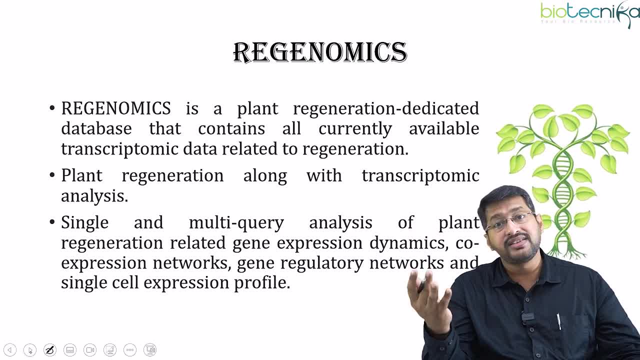 Now, as everything got, you know advanced and you know much more. you know in a futuristic sense. new terminologies such as regenomics has come into picture. Now, what is regenomics? Regenomics is mainly towards the plant biology, wherein we talk about the plant regeneration. 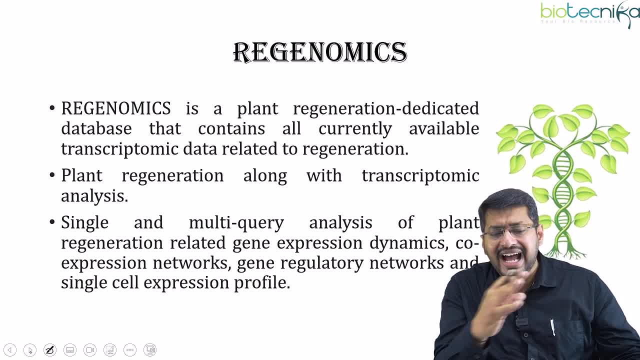 dedicated to a database Which contains entire transcriptomic data and its regenerational data. Now this becomes very, very advanced information for most of the bioinformatics data wherein we are able to clone or edit at the entire plant level, in an entire phenotypic level. 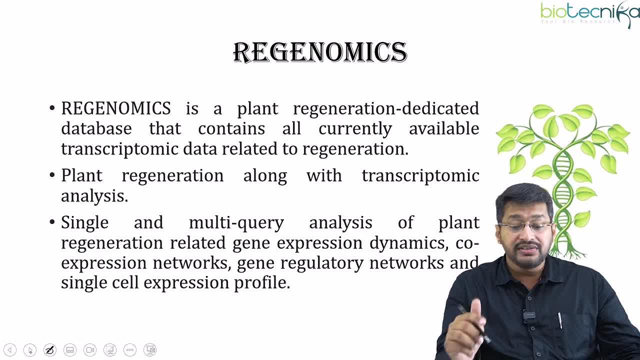 which can create genotypic variations. So hence it becomes a multi-query analysis which can lead into the expression network, gene regulatory networks and, very importantly, We can also- We can also do a single cell expression profiling of a given cell, and this is mainly towards 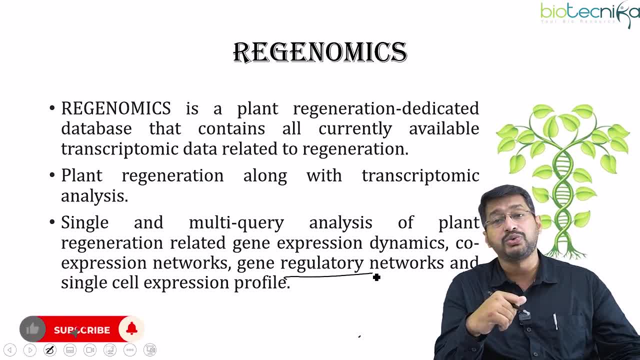 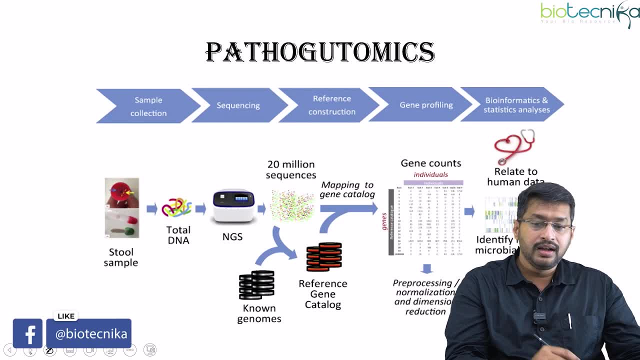 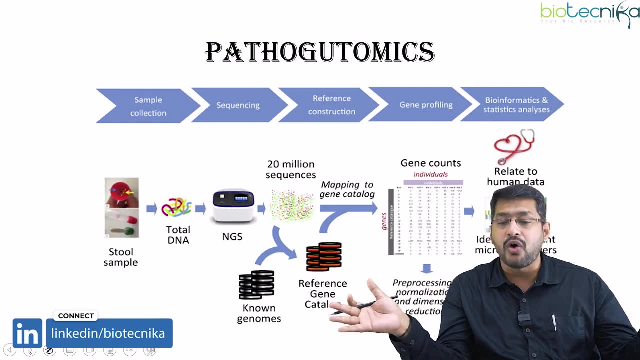 the plant biology and also sometimes also translated towards the human cells, which is called as regenomics or regeneration studies. Now, this is again new terminology which has you know, pure sciences, applied sciences and allied sciences all put together, which is called as pathoimmunogatomics. 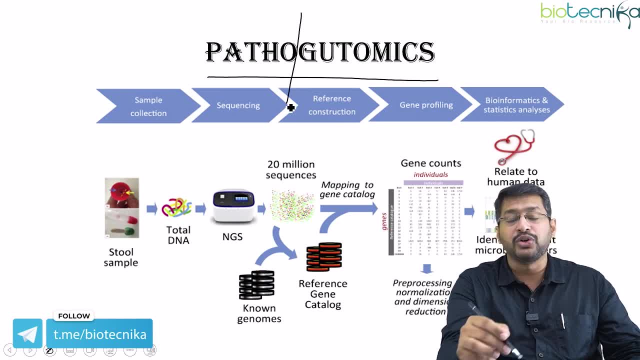 So if I decipher this particular word as patho- Patho refers to pathogen, Patho refers to pathology, and everybody now is towards microbiome. So what people say is: what you are is what you eat. So hence understanding the gut- microbiota becomes very, very important. and here comes 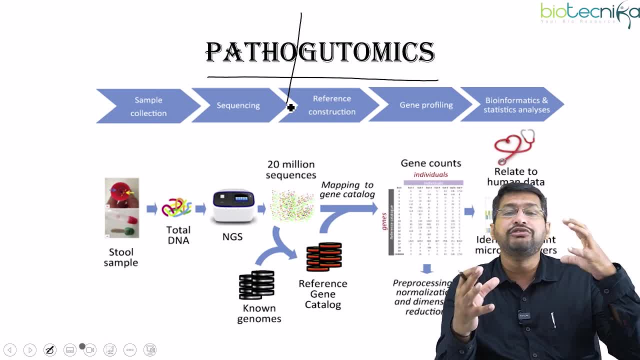 a new domain which associates gut microbiome with that of the pathological conditions of a given individual. So hence you know, you have the patho and gutto. So, and the third terminology is omics. How do you study? How do you study? 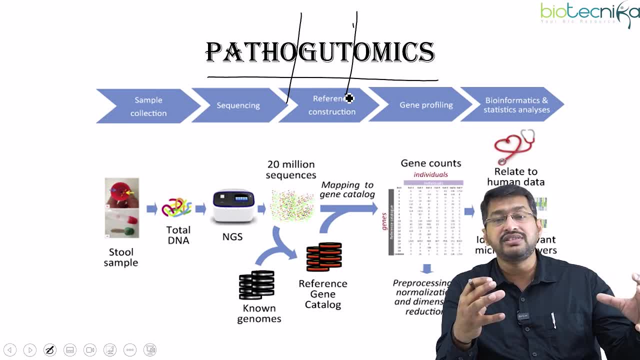 The interaction of the microbiome towards its pathogenesis or towards the health, and this is mainly by using various omic approaches, whether it could be genomics, transcriptomics, epigenetics, metabolomics or proteomics. All is put together is called as an omic approach, wherein we are talking about the pathology. 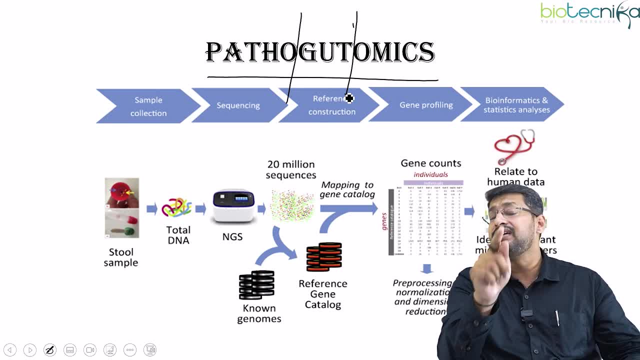 of a given individual by analyzing the gut microbiota. Here is a very important point to be remembered. so now, even if I am suffering with a disease, there are a few set of microorganisms which are responsible for it and even the reversal of the disease, wherein I can bring down the bad bacteria and bring up the good bacteria. 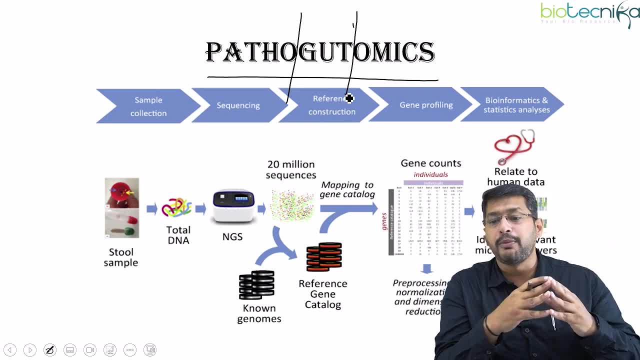 this is also possible by various components of prebiotic and probiotics. So all this put into one consortium is called as pathogatomics, and we are very happy that our group was the first group to term this terminology, which is called as pathogatomics. 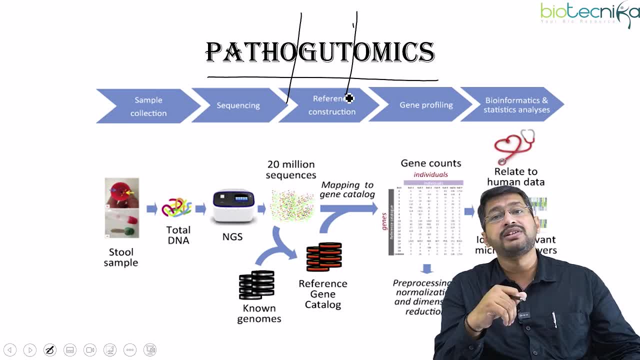 or we also call it as synthetic guttomics, Thank you. So this is a paper which has also been published in Journal of Methods in Microbiology, which has been published by Elsevier. So here the entire consortium becomes very, very important. so hence now what we need to. 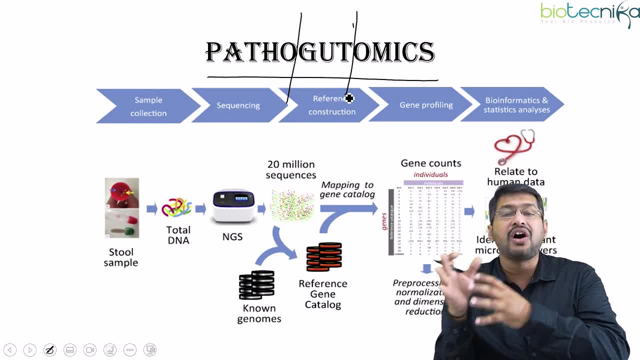 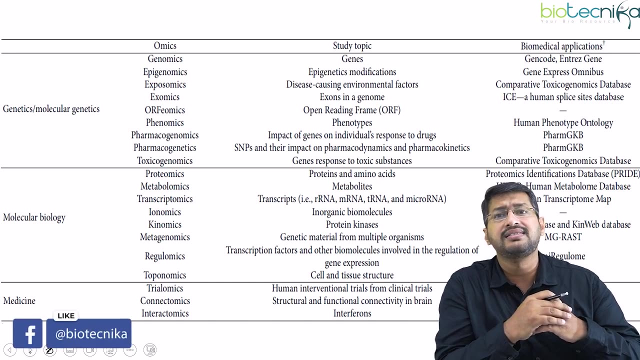 remember is it is not just the pure sciences, applied sciences or allied sciences, it is a combination, it is an amalgamation of all the three and this is leading into the generation of new, new terminologies. Now for now, For this video, I think you know understanding these new, new terminologies is sufficient. 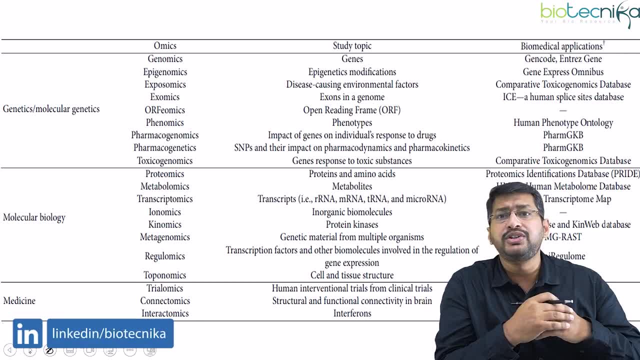 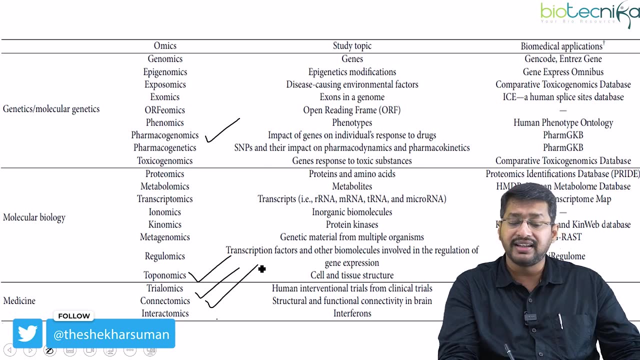 So, as a continuation video, I would also try to make you understand various newer terminologies, such as pharmacogenomics, pharmacogenetics, toxicogenomics, toponomics. then you have trilomics, then you have connectomics and then you have intromics. so all these new, new. 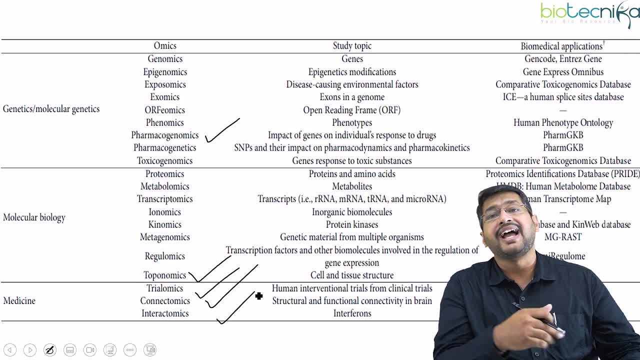 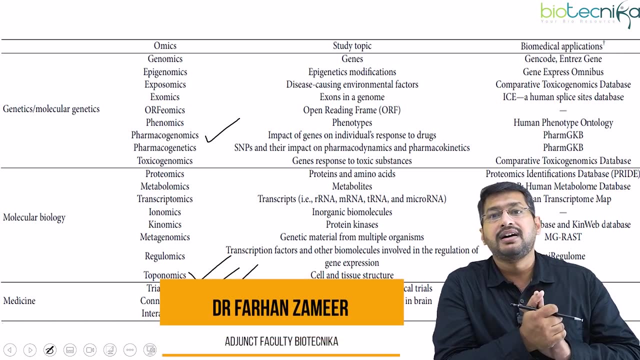 terminologies will be discussed in the next continuation video, Thank you. Thank you very much for watching and if you like all these kinds of videos, please let us know so that we can create much more content for you. so that you know, your interest creates motivation in us and this is how, together, we will make a civil society for a betterment. of science. Thank you very much. all biotechnicians, Farhan Zameer, signing off. Thank you.